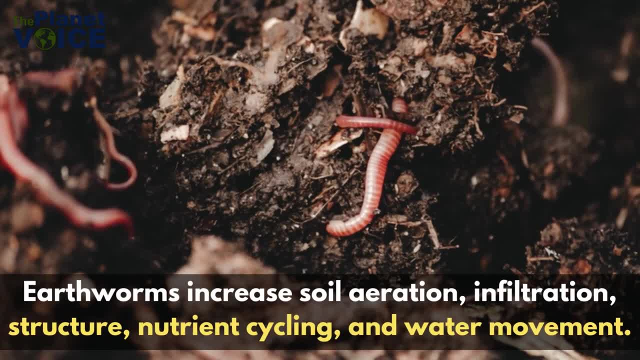 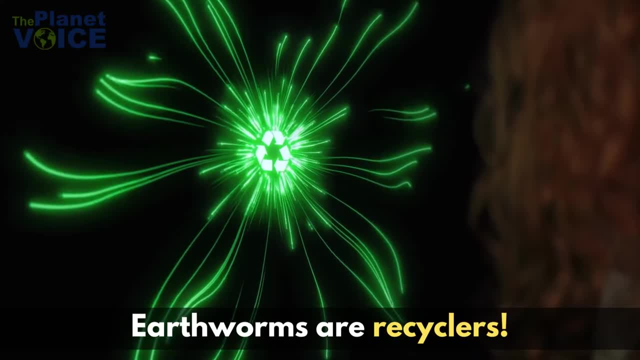 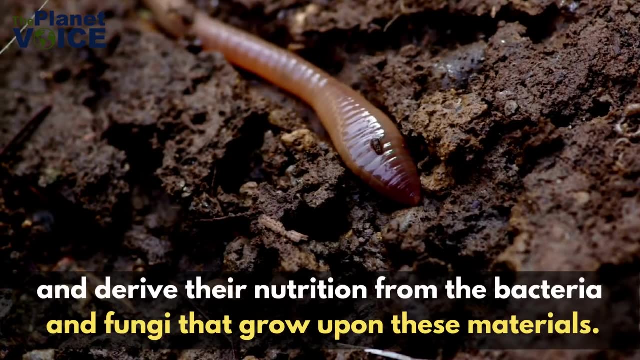 waste. Earthworms increase soil aeration, infiltration structure, nutrient cycling and water movement. Earthworms are recyclers. They are major decomposers of dead and decomposing organic matter and derive their nutrition from the bacteria and fungi that grow upon these. 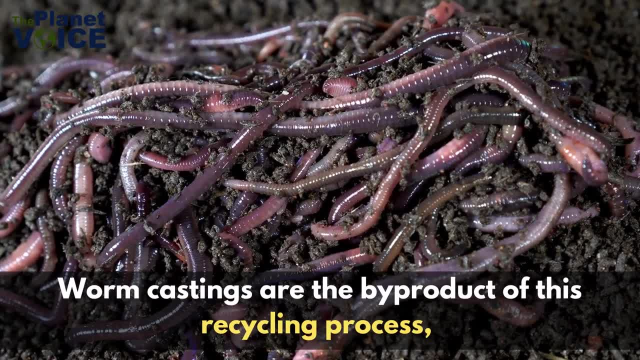 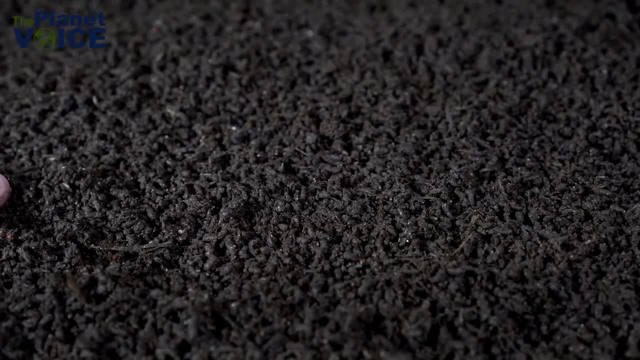 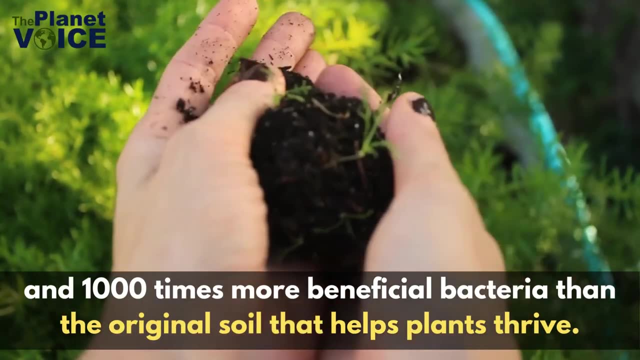 materials. Worm castings are the byproduct of this recycling process, which can occasionally be seen as small mounds on top of the soil. Their casts can contain five times more nitrogen, seven times more phosphorus and one thousand times more beneficial bacteria than the original soil. that helps plants thrive. 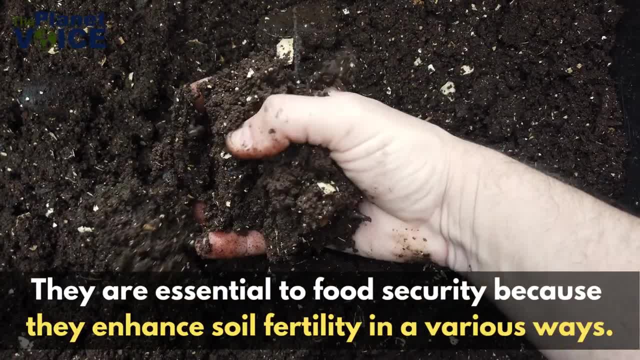 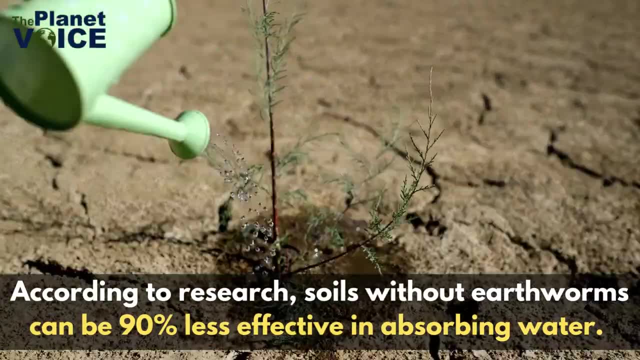 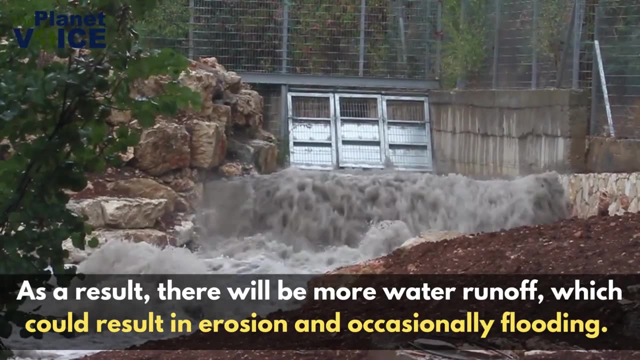 They are essential to food security because they enhance soil fertility in a various ways. According to research, soils without earthworms can be 90% less effective in absorbing water. As a result, there will be more water runoff, which could result in erosion and, occasionally, 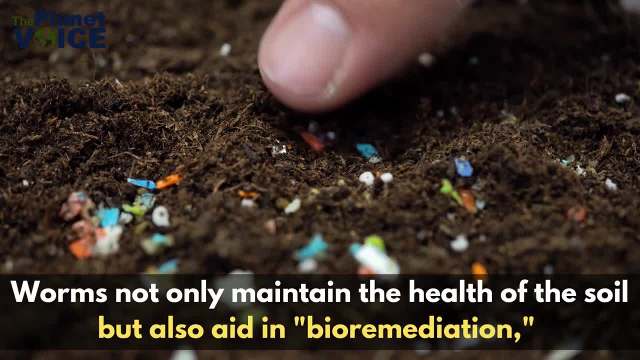 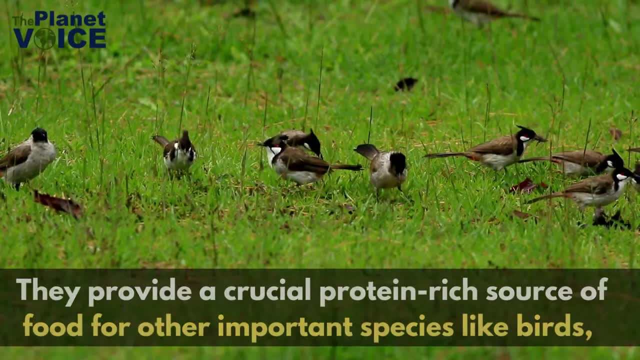 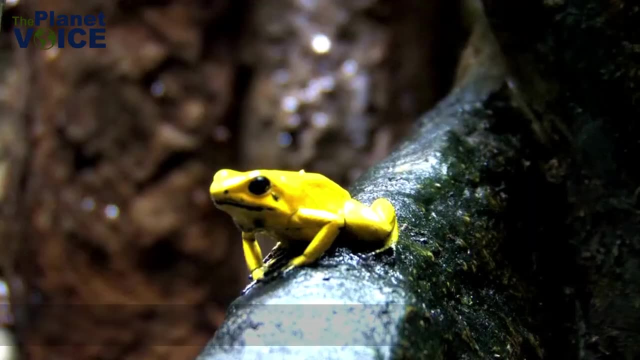 flooding Worms not only maintain the health of the soil, but also improve soil health. Earthworms also aid in bioremediation, which helps clean up contaminated land. They provide a crucial protein-rich source of food for other important species like birds, hedgehogs. 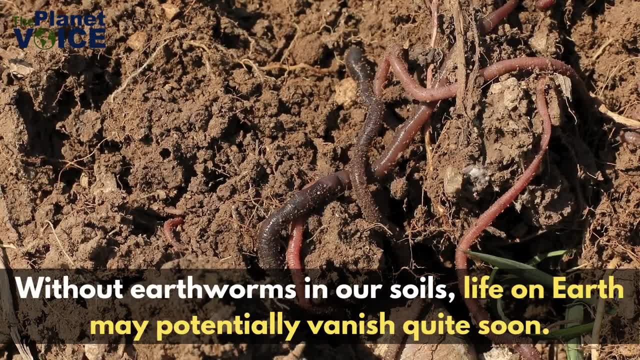 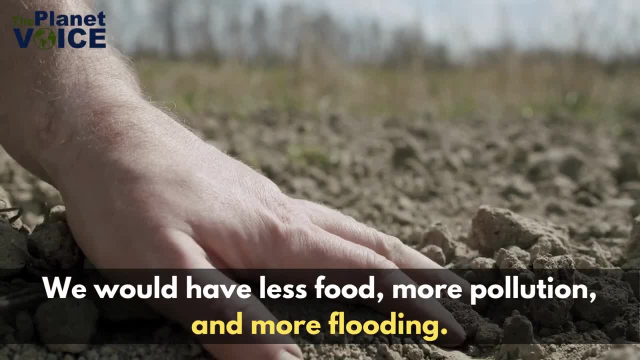 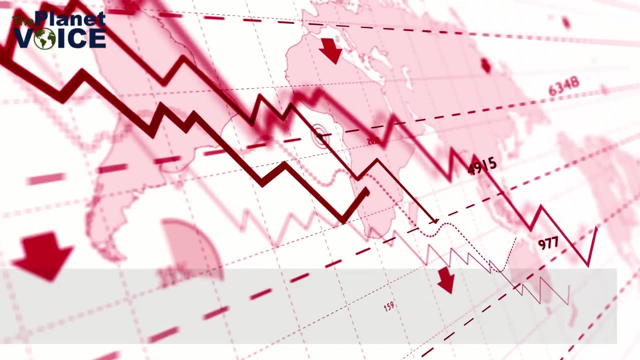 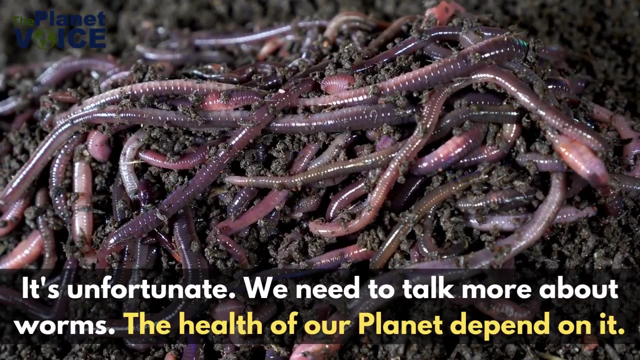 and frogs. Without earthworms in our soils, life on earth may potentially vanish quite soon. We would have less food, more pollution and more flooding. Yet, despite their importance, earthworms are under serious threat. Yet, unlike other creatures, the decline of worms rarely makes the news. It's unfortunate. 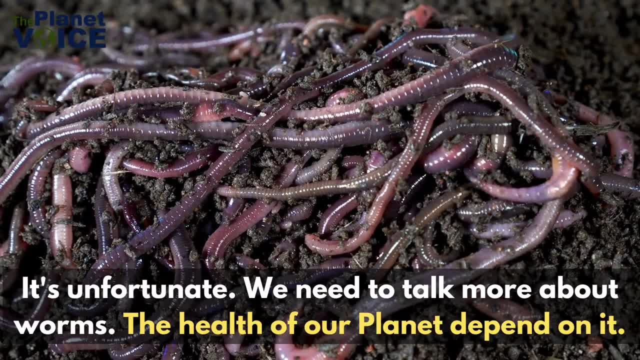 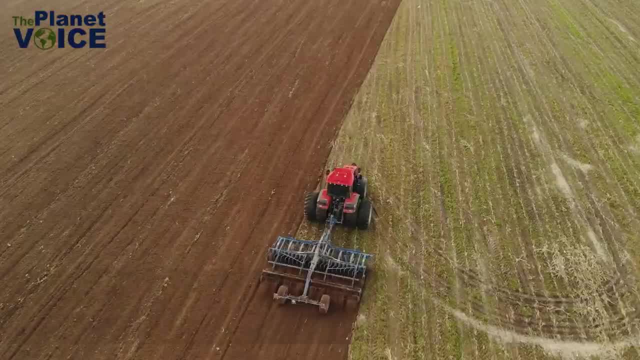 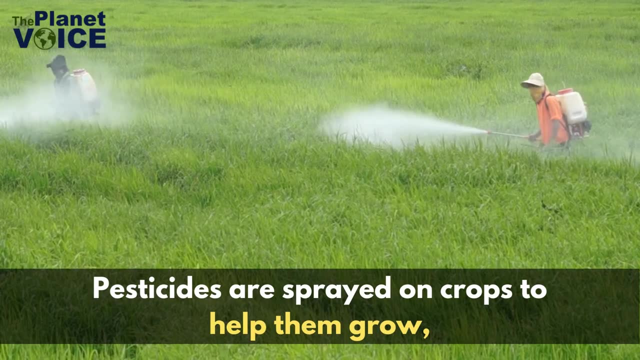 We need to talk more about worms. The health of our planet depend on it. Earthworm populations all across the world are suffering greatly from the digging, stirring and turning of soil caused by conventional plowing in tillage farming. Pesticides are 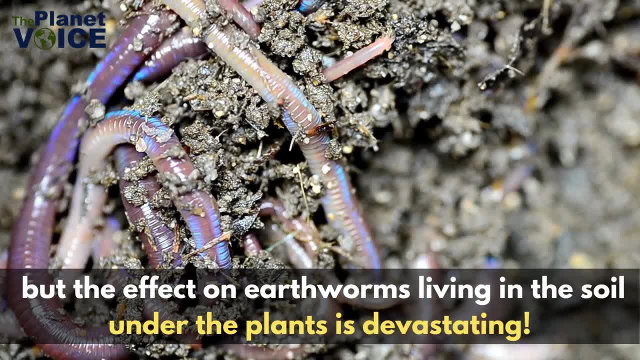 sprayed on crops to help them grow. but the effect on earthworms is very small. They can only be found on the surface of the earth. They can only be found on the surface of the earth. They can only be found on the surface of the earth. They can only be found on the